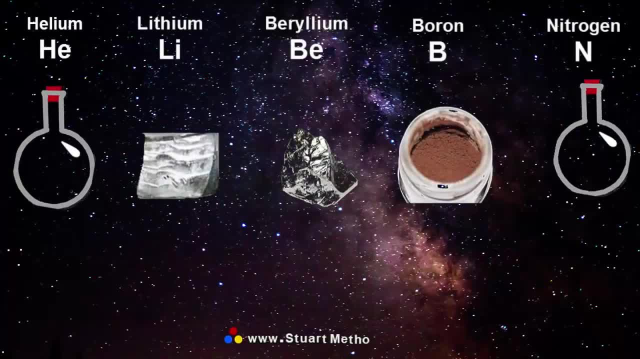 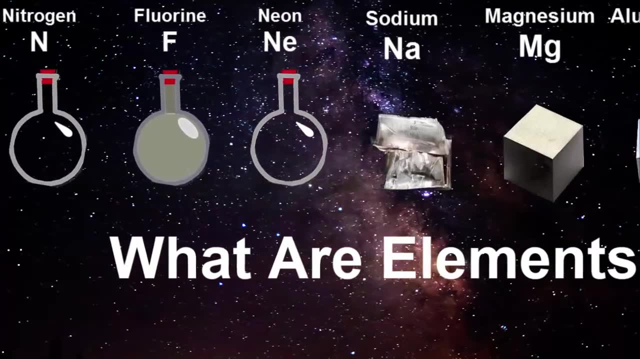 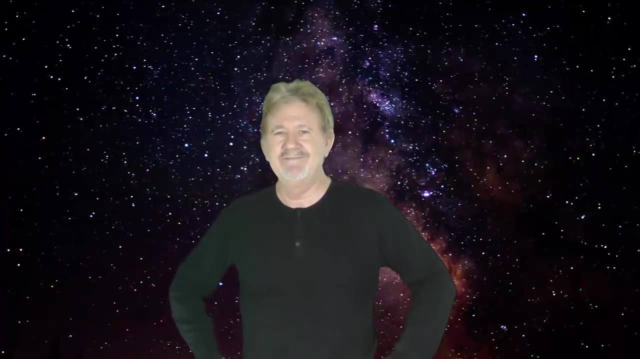 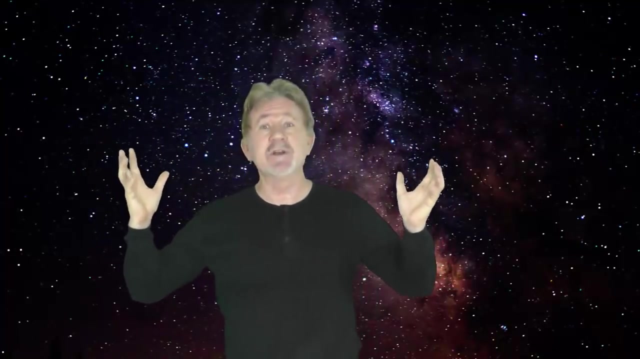 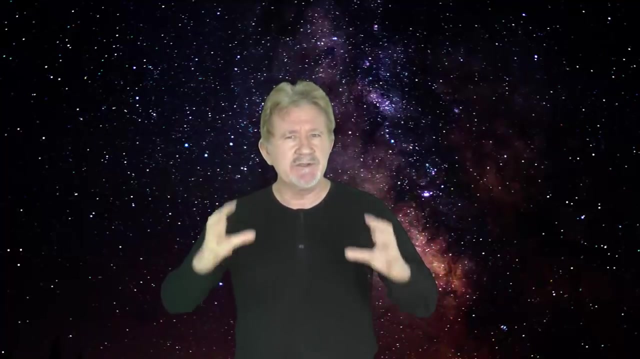 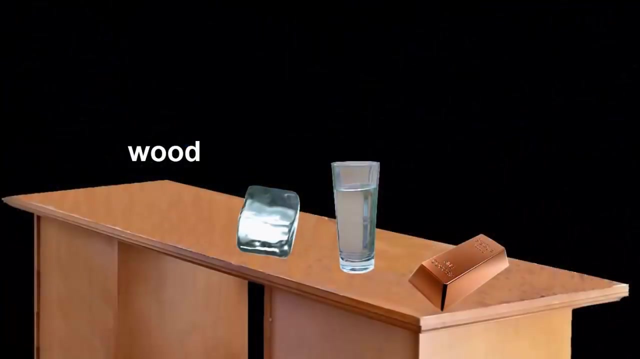 All the things in the universe are made from just 92 different kinds of atoms. Atoms are too small to see with our eyes, so we can only see the substances that they make. Here are four substances: Wood from a desk, a lump of glass, water and an ingot. 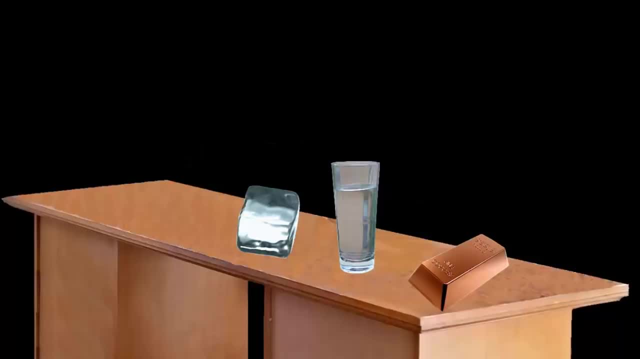 of copper, But to see their atoms we'd need to magnify them to make them look a billion times bigger. Let's do that. Normally the different kinds of atoms are all mixed up and joined to other atoms and it's unusual to find one kind of atom all on its own. To tell the atoms apart, we've 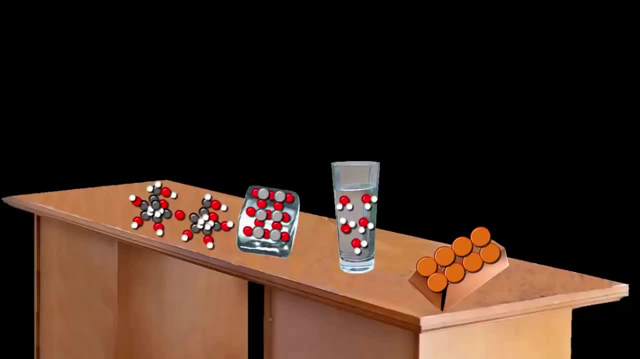 made an atom code with different coloured balls and one or two letters. The little white ones show hydrogen atoms, with letter H, The black one's, carbon oxygen's are red, silicon's grey and copper is orange. Notice that oxygen is in three different substances here: Wood, glass and water. 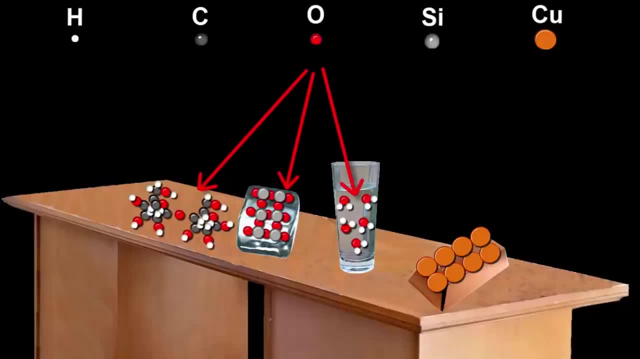 Which look and feel very different to each other, And hydrogen is in both wood and water. The same atoms can make completely different substances when they're put together in different ways. Now we're going to pull apart all of the atoms. Now we're going to pull apart all of the atoms. 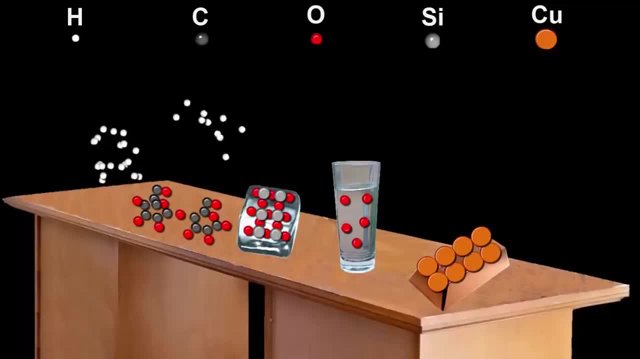 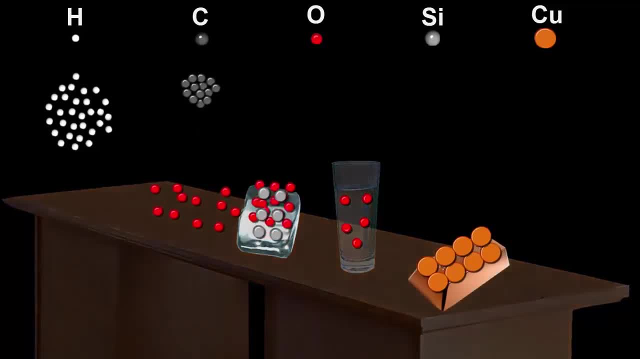 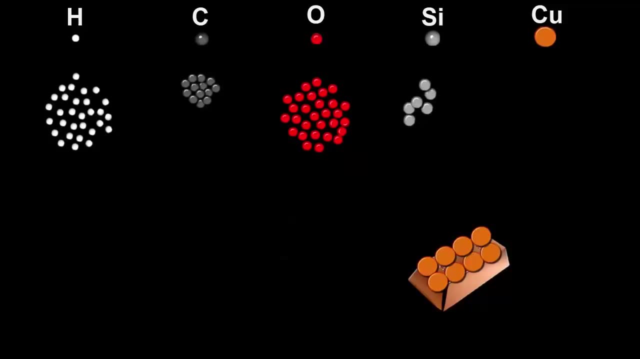 The carbon's here, Oxygen's here, Silicon's here And copper's here. We can't pull the atoms apart. We can't pull the atoms apart. We can't pull the atoms apart. So they're now as simple as they can get. 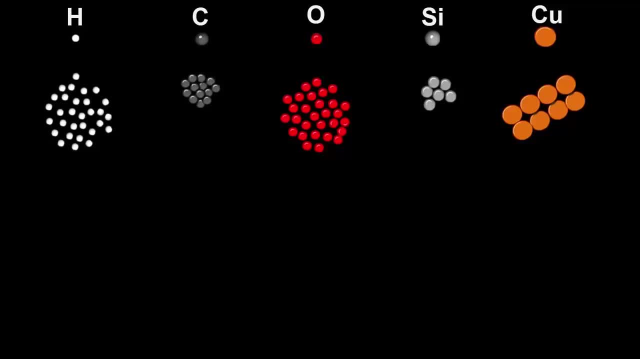 These five piles of atoms make substances too, But they look and feel different when they're all on their own. A collection of hydrogen atoms will make a colourless gas, So we'll have to catch them in a jar and put a lid on it so it doesn't escape. 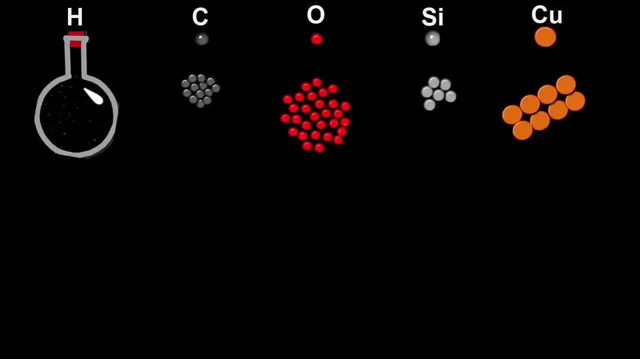 We'll now shrink the atoms back to their real size and out of sight. We'll now shrink the atoms back to their real size and out of sight. A collection of carbon atoms will make a black, solid. Oxygen atoms will also make a colourless gas. 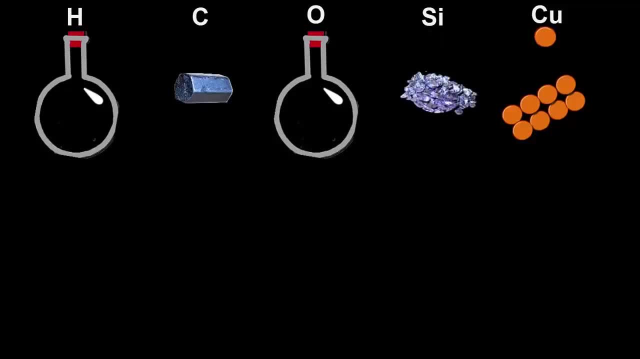 And silicon atoms make a shiny grey solid. Copper atoms make a shiny orange solid. By the way, the colour of the substance isn't necessarily the same as its atoms. We've just done that to make it easier to follow. These substances containing only one kind of atom are as simple as they can get. 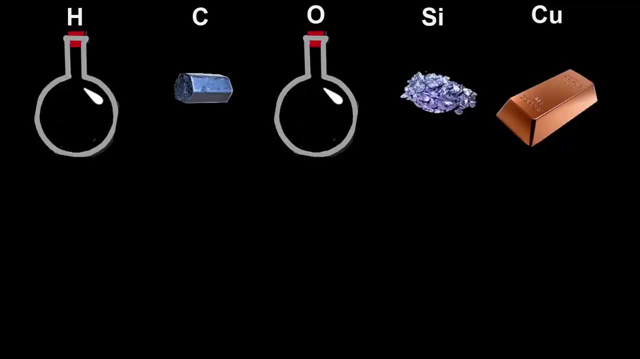 Because they can't be separated into any more kinds of atoms, So they're given a special name: Elements. An element is a substance made of only one kind of atom. Strictly speaking, an element refers to the substance that you can see and touch. 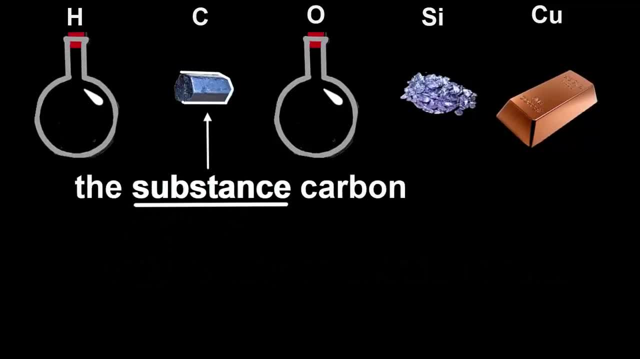 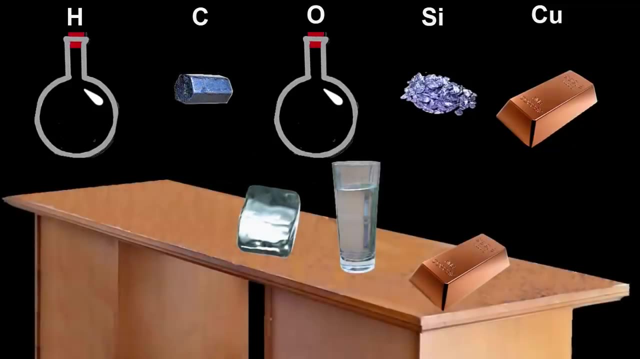 Such as the chunk of carbon. that's made of trillions of trillions of carbon atoms, But sometimes we talk about a single atom of carbon as being an element too. And did you notice that one of the substances on the desk that we started with had only one kind of atom in it? 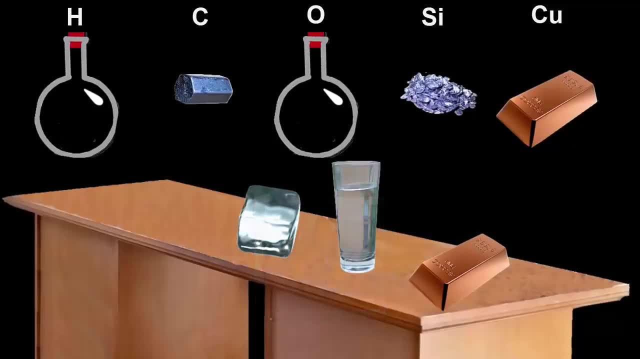 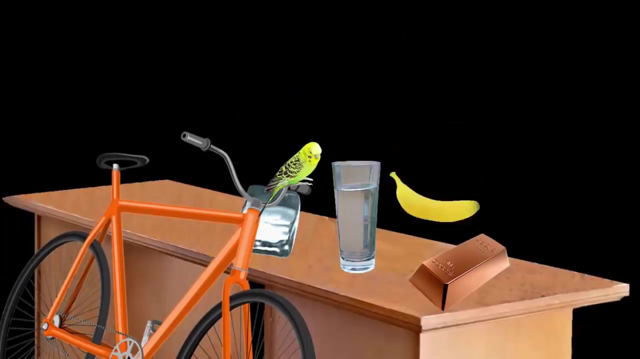 Which one Copper? Copper was already an element before we pulled it apart and put it back together again. For fun, let's throw in more objects at the bottom of our screen: A bike, A budgie, A banana And a ball.